recuerdaidnizno iruvio and adultsize sedutum. Water is excreted in theänder sulfidebank отсor bedtime syrou and bubbles are released in the puedo of de plomo. 快der staat подß pun. Flying does not do it, most likely, but the use of this method Esse if. 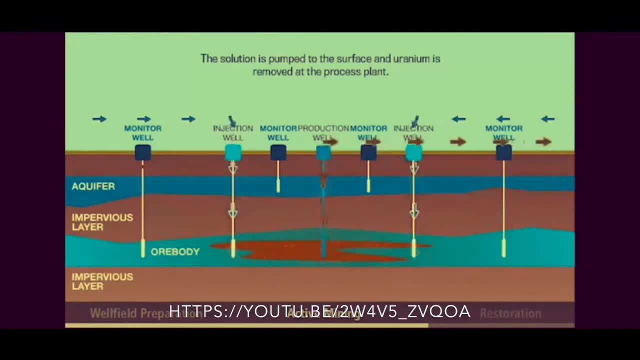 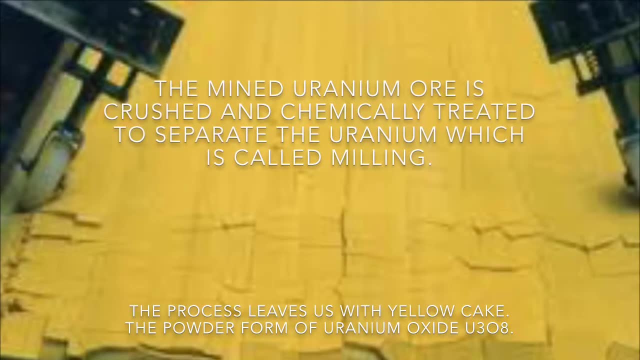 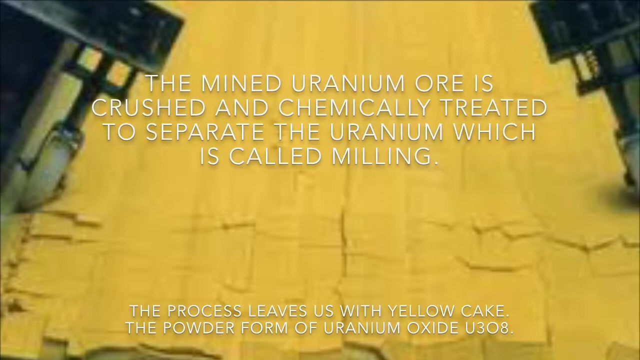 she slut in the near near future of more fast About. the radically concentrated oxidation is pumped to the surface and uranium is removed at this process plant. The mined uranium ore is crushed and chemically treated to separate the uranium, which is called milling. The process leaves us with yellow cake, the powder form of uranium oxide. The second stage is conversion of. 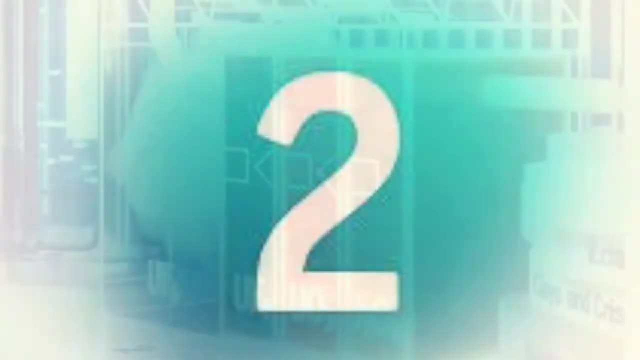 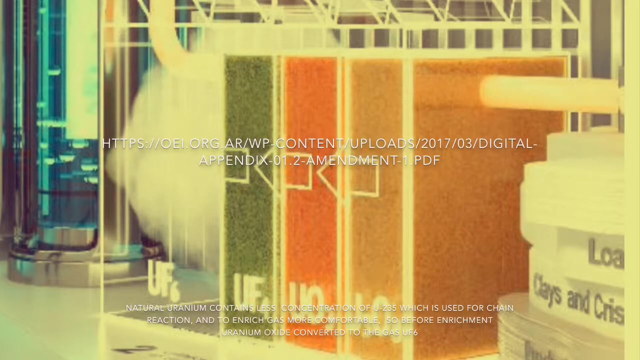 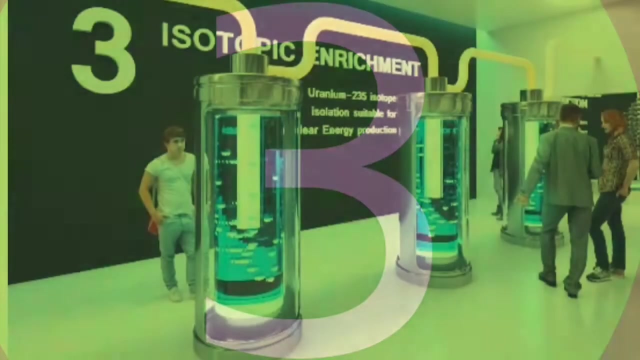 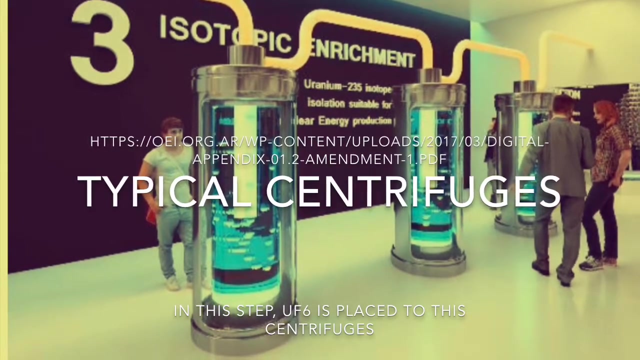 uranium powder to the gas. Natural uranium contains less concentration of uranium 235, which is used for chain reaction and to enrich gas is more comfortable. So before enrichment, uranium oxide converted to the gas. This is conversion. The third step is enrichment. In this step, uranium hexothalite is placed in these centrifuges. Two main isotopes of uranium are: 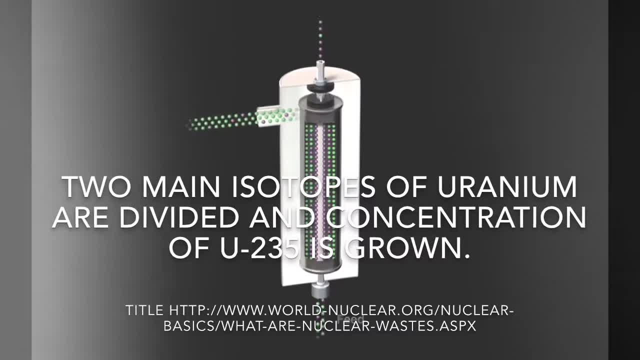 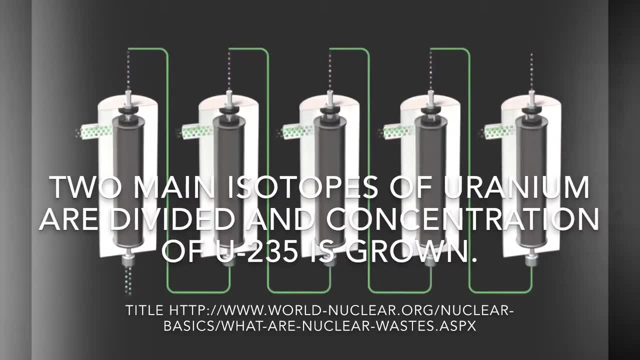 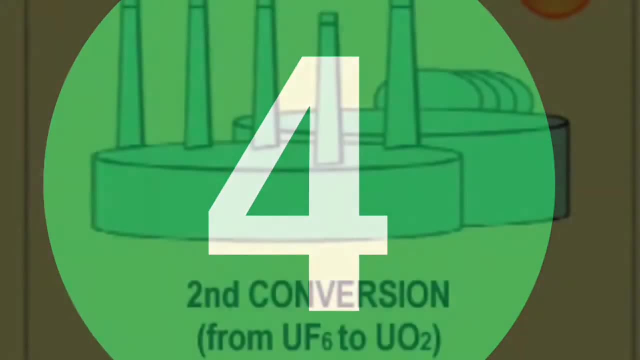 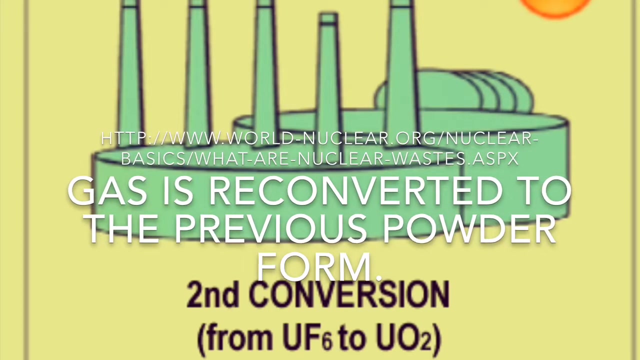 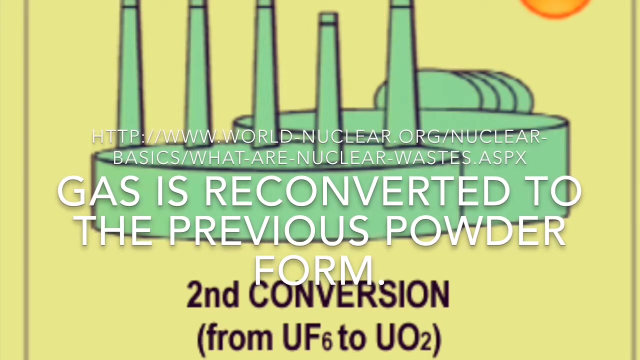 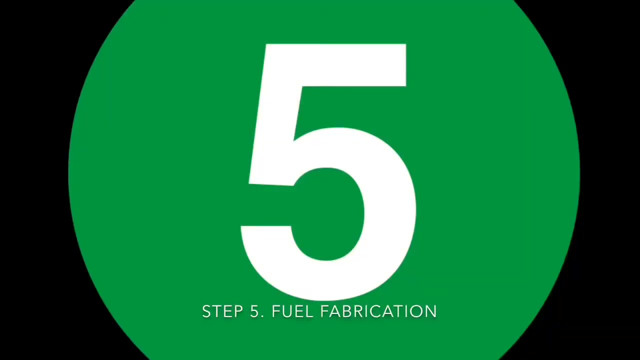 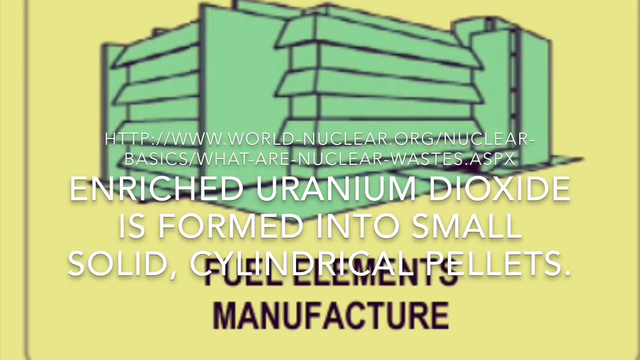 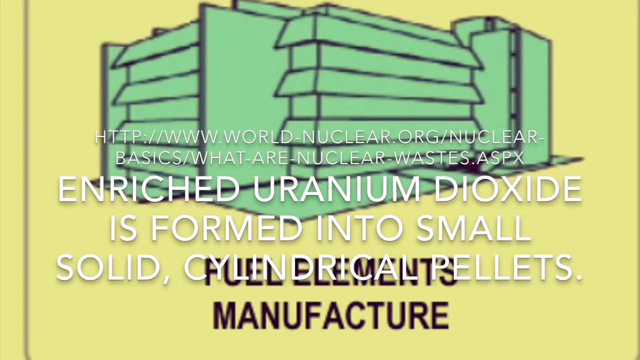 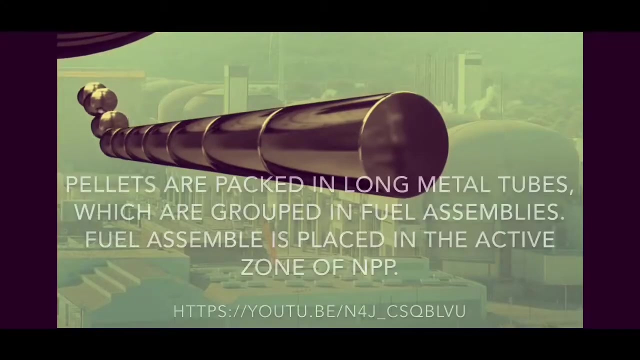 divided and the concentration of uranium 235 is grown. Step 4 reconversion Gas is reconverted to the previous powder form. Step 5 fuel fabrication In the steppe enriched and uranium dioxide is formed into oggiative Étand small solid cylindrical pellets. 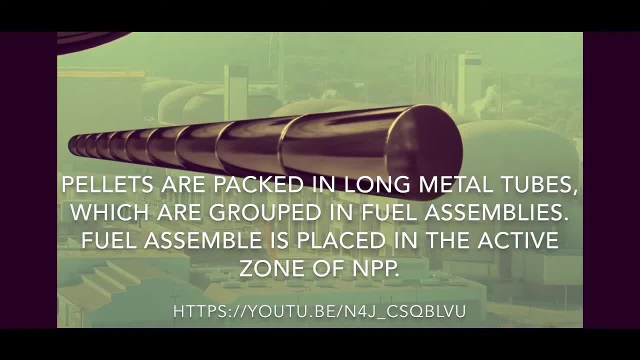 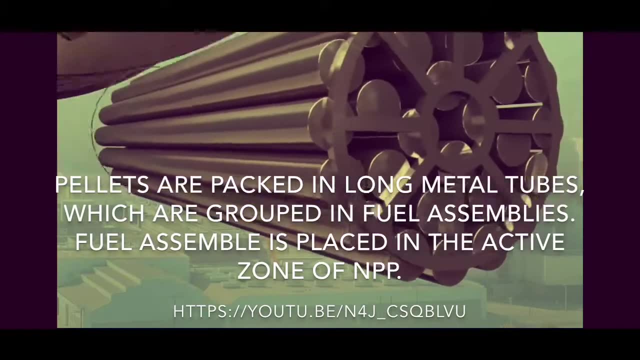 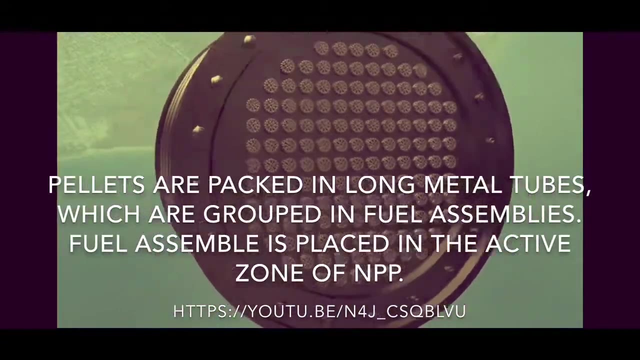 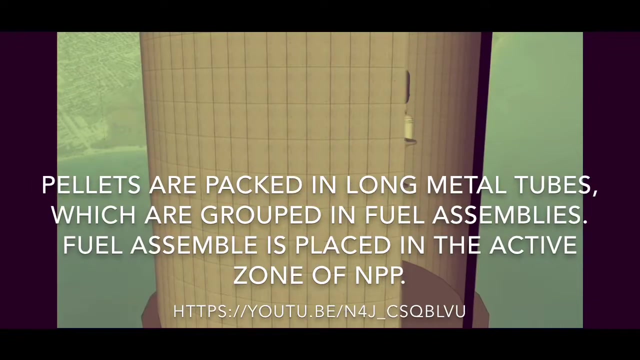 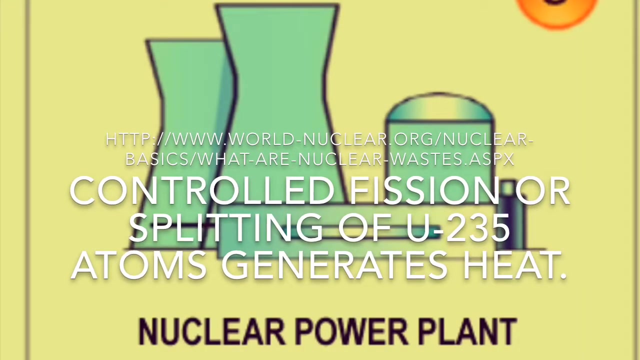 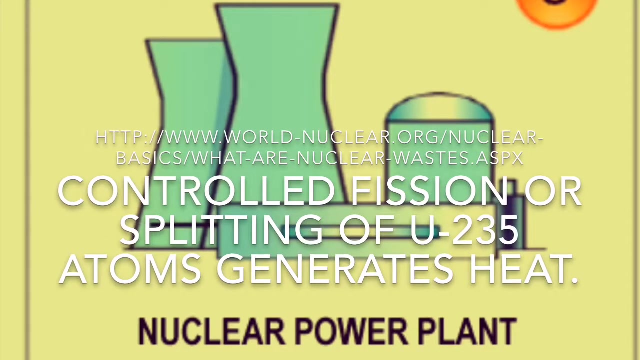 Uranium pellets are packed in long metal tubes, which are grouped in fuel assemblies. Then this fuel assemblies is located in the active zone of nuclear power plant. Controlled fission or splitting of uranium-2,3,5 atoms generates heat- Heat. 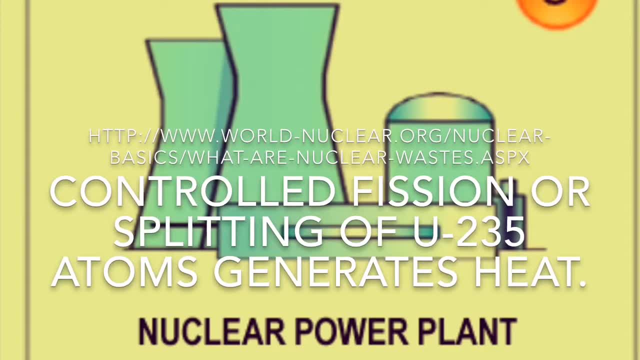 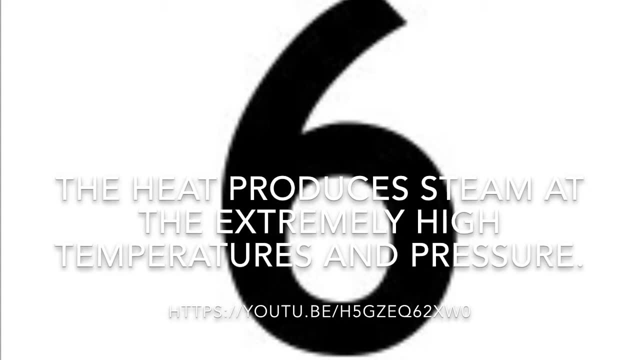 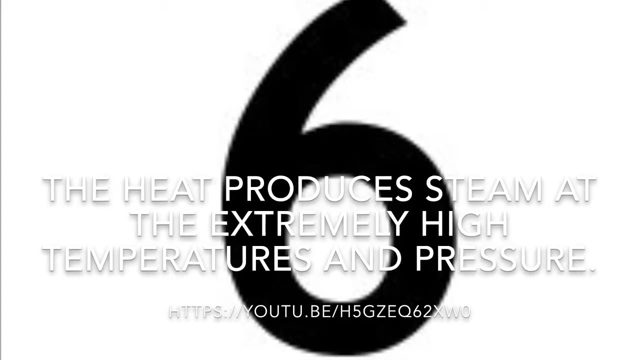 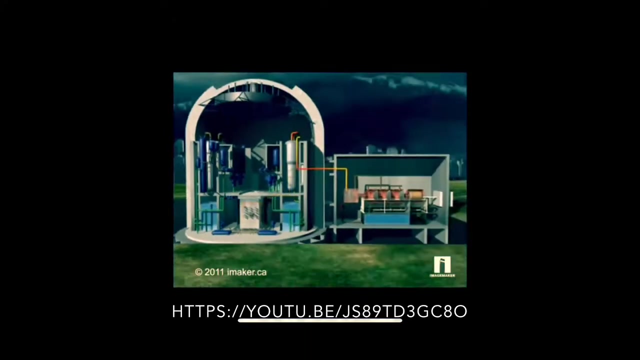 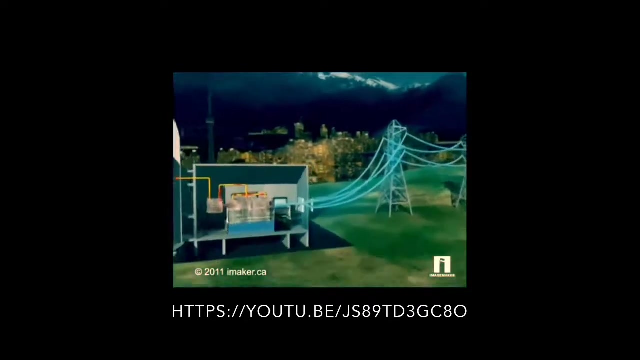 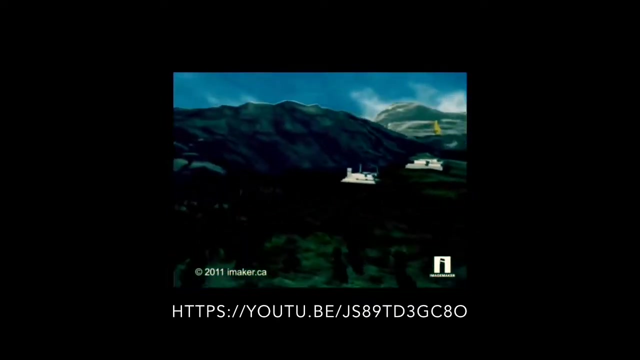 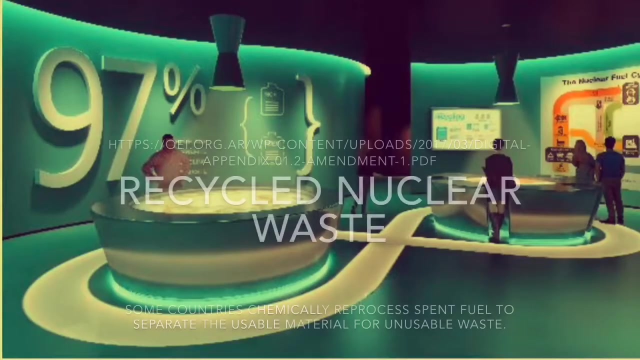 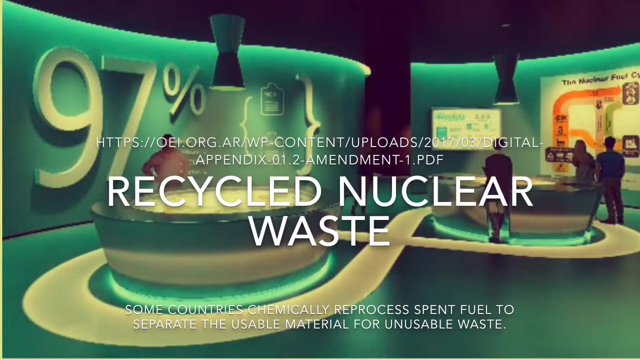 The heat produces steam at the extremely high temperatures and pressure. The steam spins turbine to generate electricity. Heat generates more energy. Step 7. Nuclear waste management, Recycling. Some countries chemically reprocess spent fuel to separate usable material from unusable. 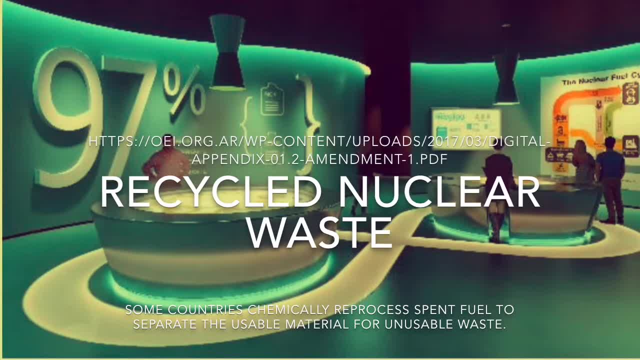 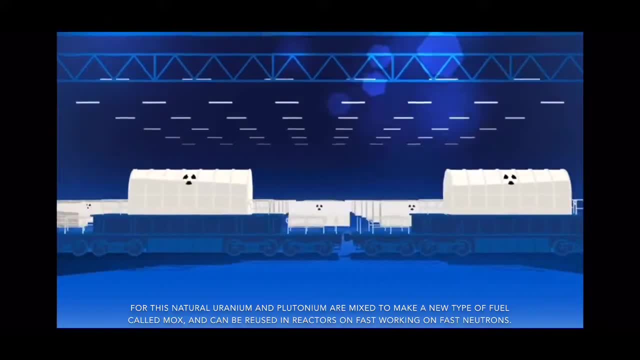 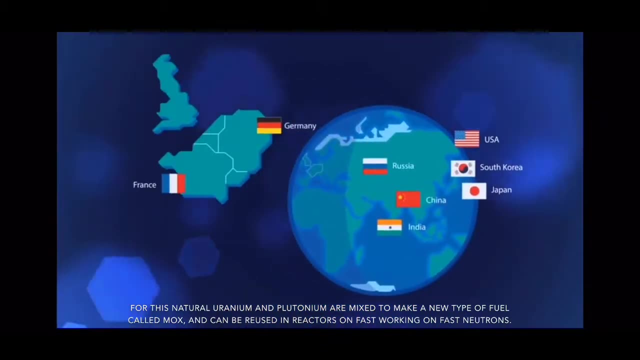 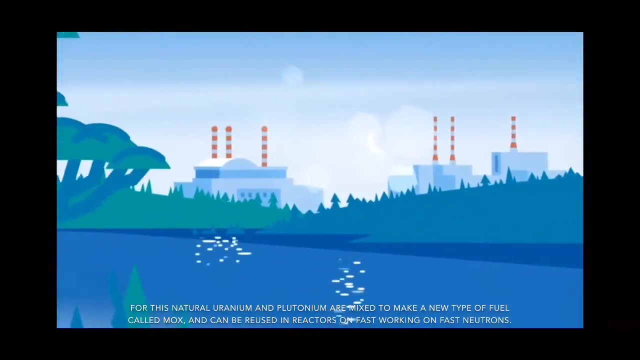 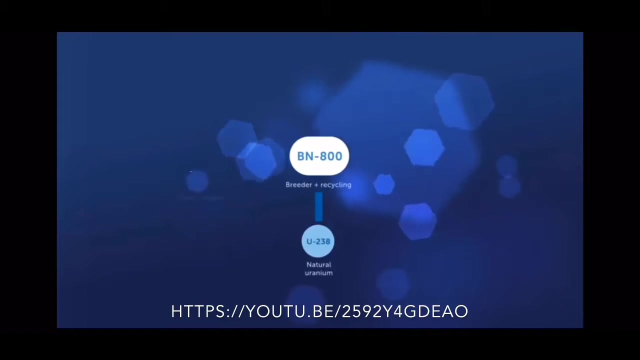 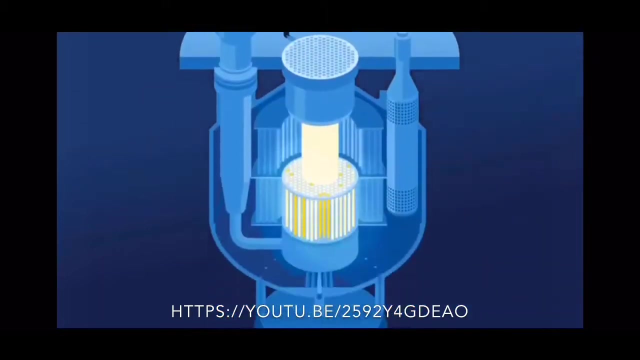 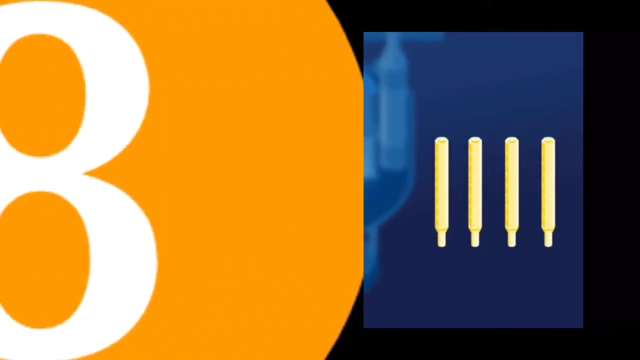 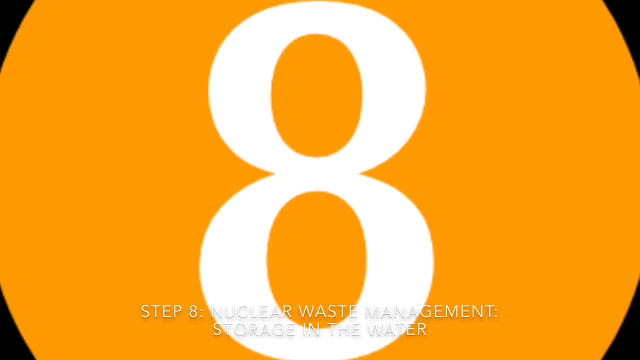 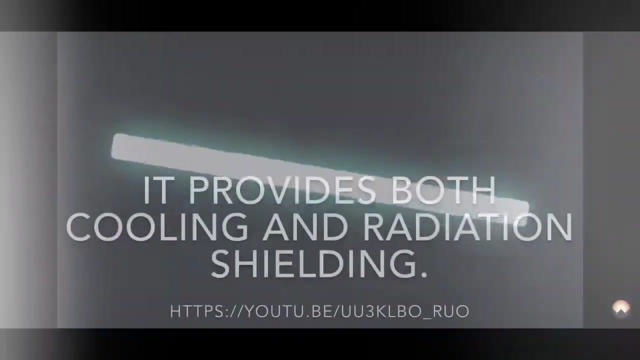 waste. For this, natural uranium and plutonium are mixed to make a new type of fuel called MOX and can be reused in reactors on fast working on fast neutrons. Step 8. Nuclear waste management Storage in the water. This is the first short storage step that is stored under water, which provides both cooling and radiation shielding. 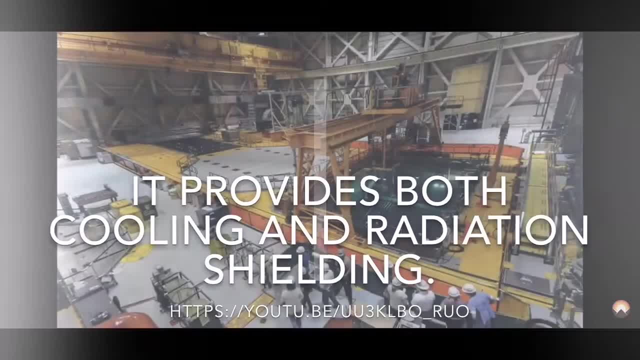 This is the first short storage step that is stored under water, which provides both cooling and radiation shielding. This is the first short storage step that is stored under water, which provides both cooling and radiation shielding. Storage in the water will last 3-5 years. 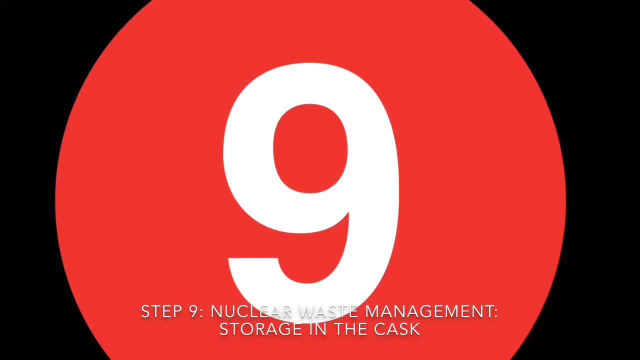 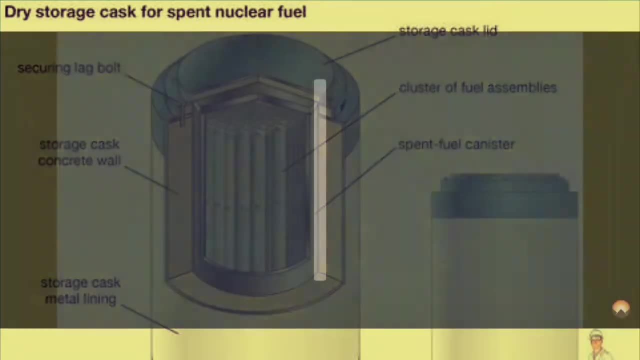 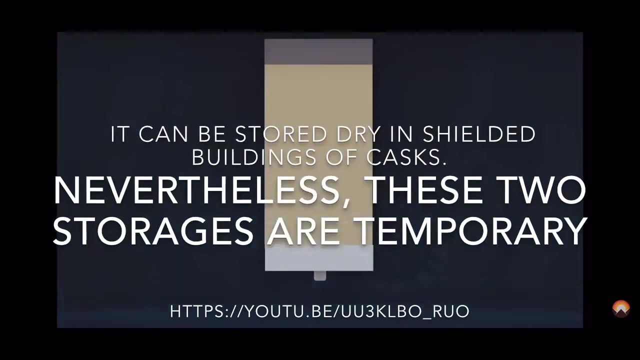 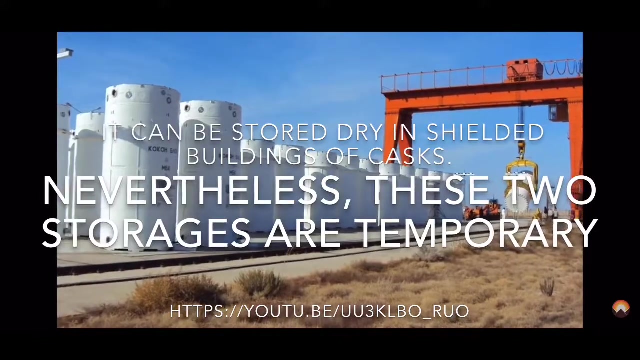 Step 9. Storage in the casks. Step 9. Storage in the casks. It can be stored dry in shielded buildings of casks. Nevertheless, these two storages are temporary. The cost is not fixed, so we do the sewing one by one. 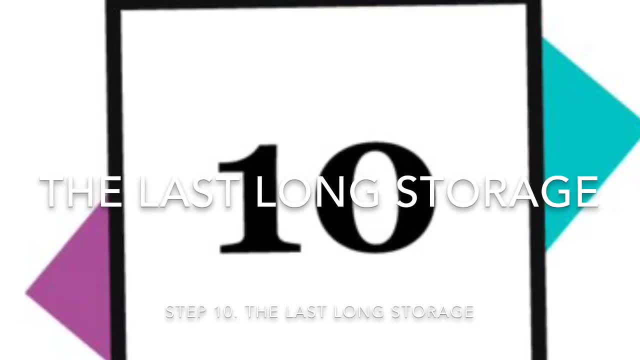 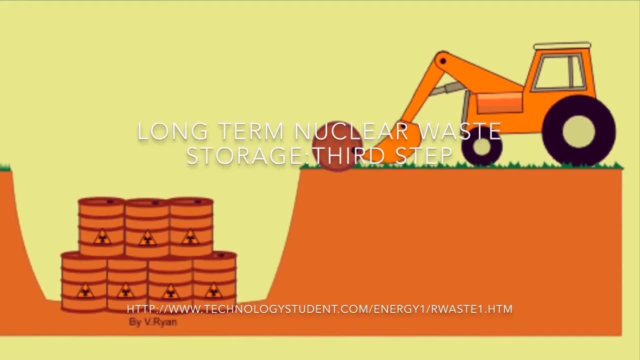 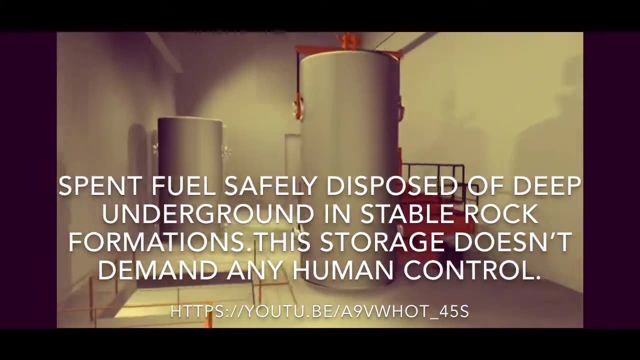 Step 9. Last: long storage. In this step, spent fuel locally stored under water is safely disposed of deep underground in stable rock formations. In this step, spent fuel locally stored under water is safely disposed of deep underground in stable rock formations. 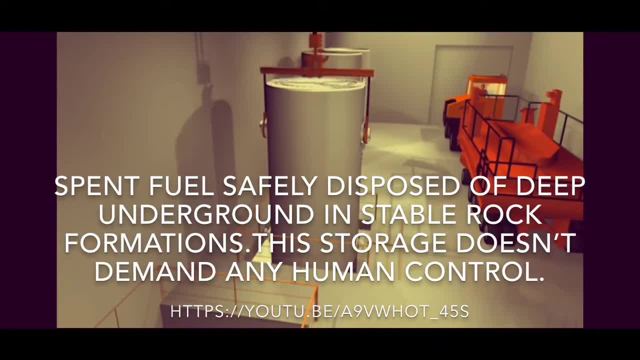 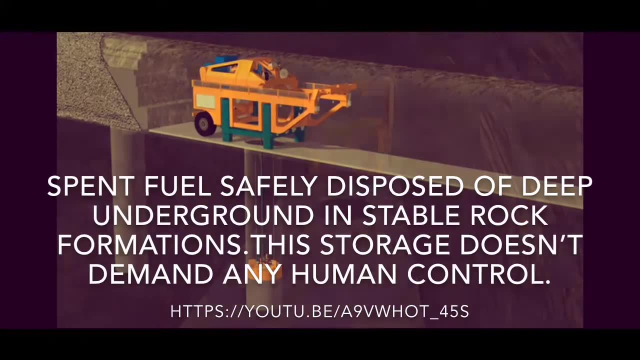 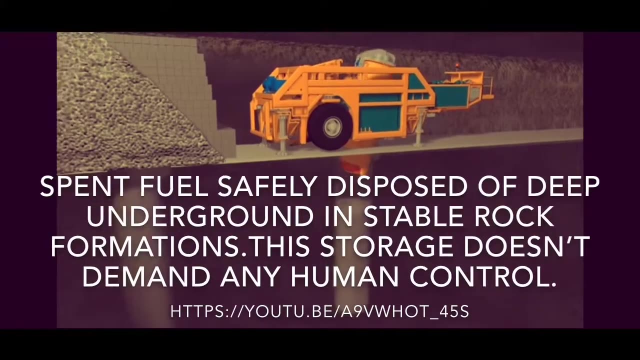 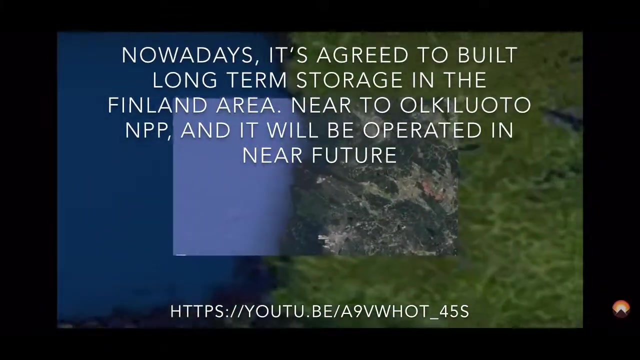 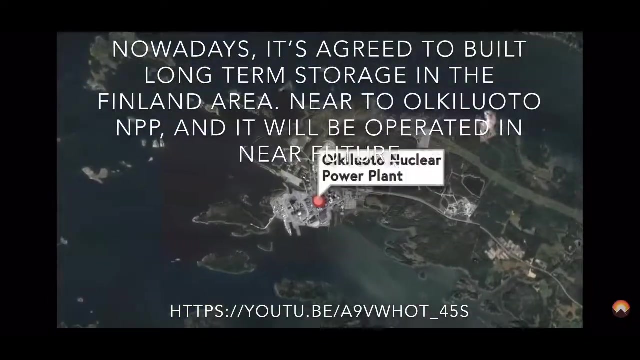 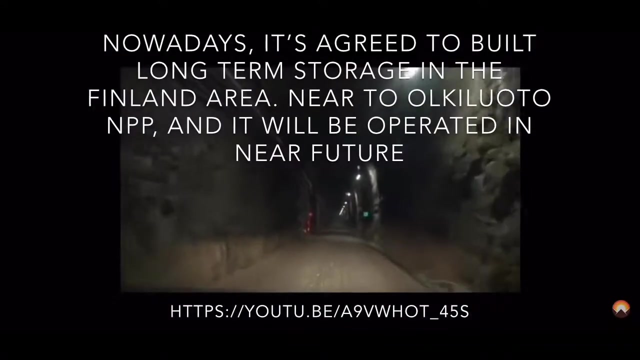 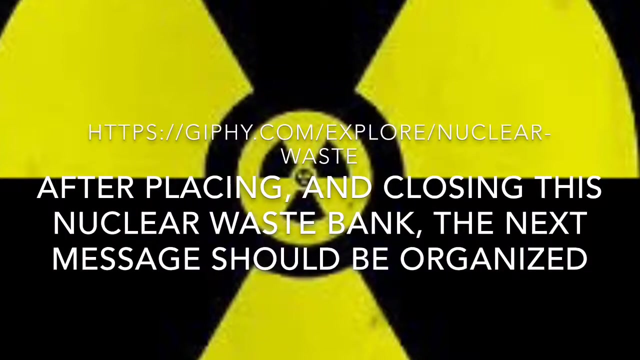 This kind of storage system doesn't demand any human control. Nowadays it's agreed to build long-term storage in the Finland area near to Olkioloto nuclear power plant, and it will be operated in near future. After placing and declosing this nuclear waste bank, the next message should be organized. 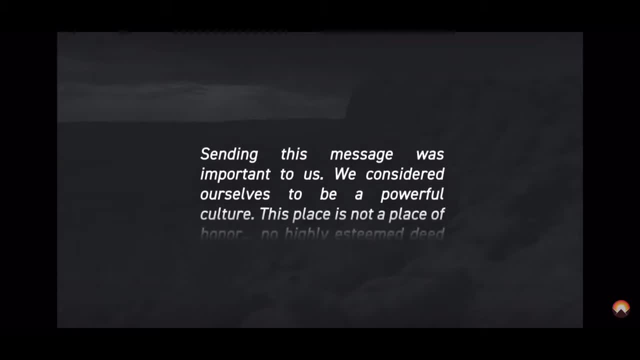 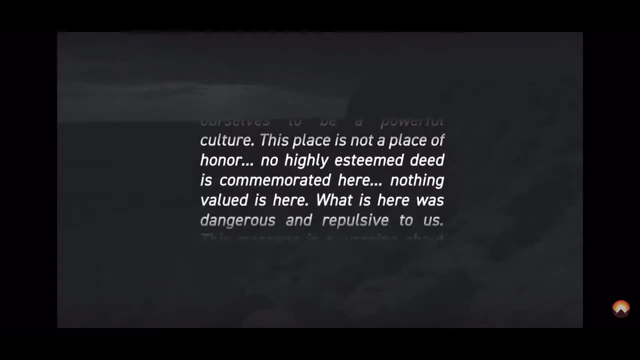 Sending this message was important to us. We considered ourselves to be a powerful culture. This place is not a place of honor. no highly esteemed deed is commemorated here. nothing valued is here. What is here was dangerous and repulsive to us. This message is a warning about danger. 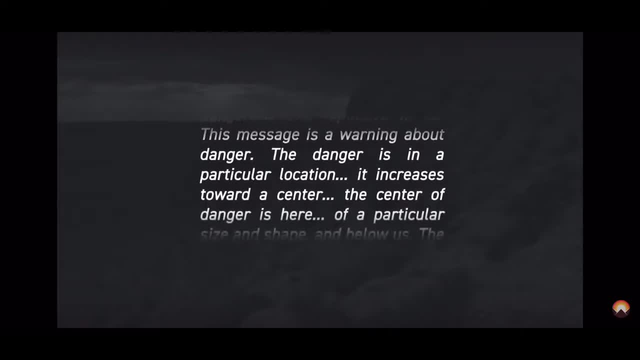 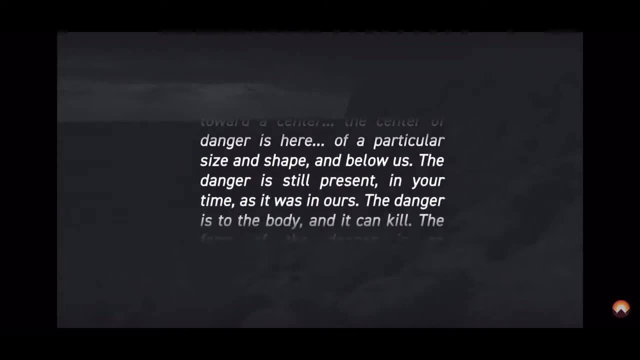 The danger is in a particular location, It increases towards the center. The center of danger is here of a particular size and shape, and below us The danger is still present in your time as it was in ours. The danger is to the body and it can kill. 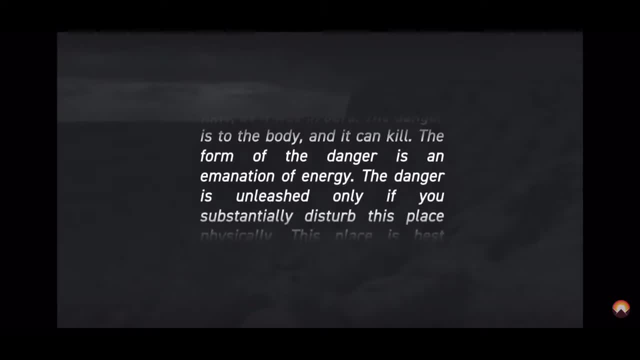 The form of the danger is an emanation of energy. The danger is unleashed only if you substantially disturb this place physically. This place is best shunned and left uninhabited. The idea would be to translate a message like this into every United Nations language—.